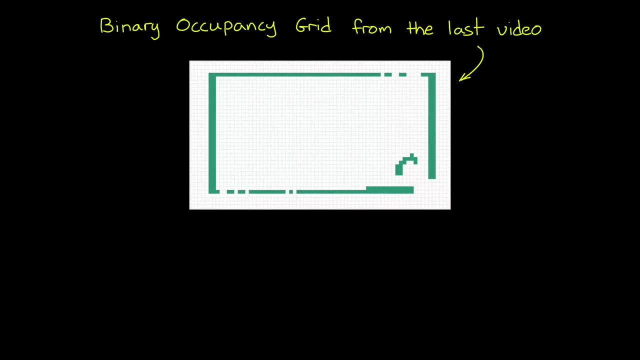 In the last video, we covered simultaneous localization and mapping and, as the name suggests, we ended up with a map of the environment in the form of a binary occupancy grid. Now for this video, we're going to explore some of the ways that we can use a map like this. 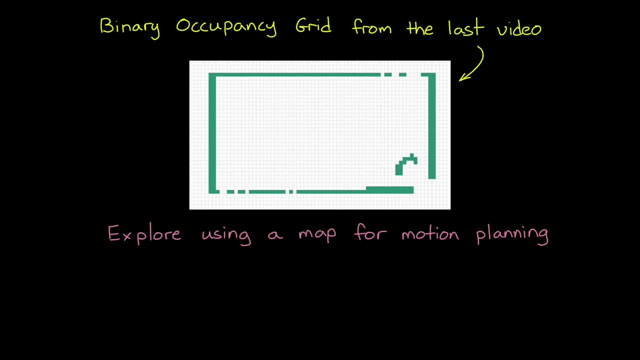 for motion planning, That is, finding a trajectory through the environment that connects a robot's starting state to some goal state. And we're going to briefly cover what motion planning means and how we can use a graph to solve this planning problem. And then we're going to cover two popular 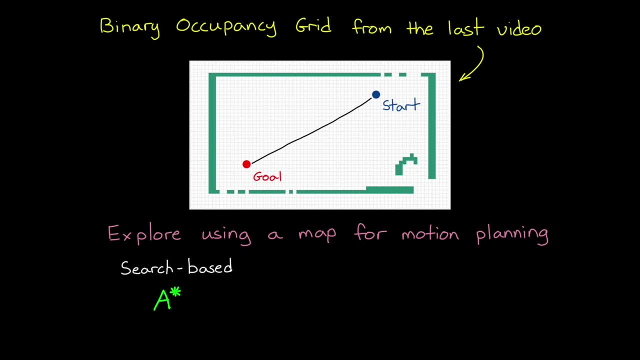 approaches for creating that graph: Search-based algorithms like A star and sampling-based algorithms like RRT and RRT star, And I think this video will sort of nicely set a base understanding of how we can use graphs to plan a trajectory through a known environment. And 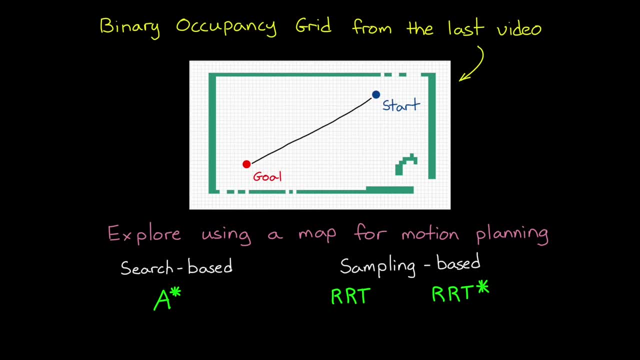 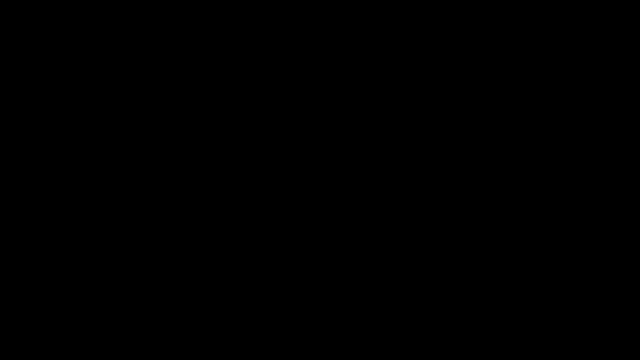 it's something on which you can build when you go out and learn more about these planning methods, So I hope you stick around for it. I'm Brian, And welcome to a MATLAB Tech Talk. We want to find a path from a starting pose to a goal pose, And if we're talking about a robot, 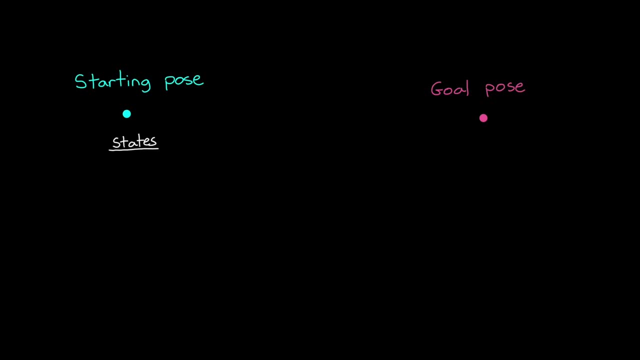 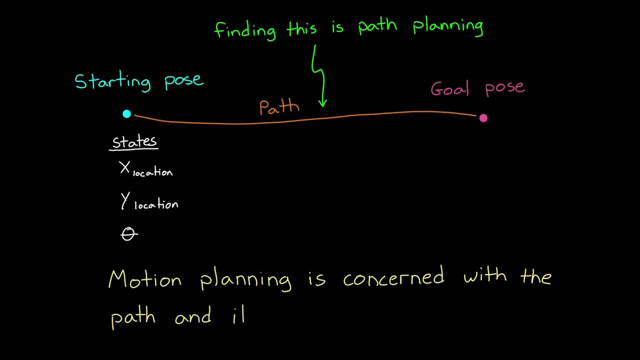 a subset of the larger motion plan. Now, path planning is just a subset of the larger motion planning. problem: With motion planning we're not just concerned with the sequence of poses, but also their derivatives, like velocity, acceleration, rotation rate and so on. So with motion planning we're trying to dictate. 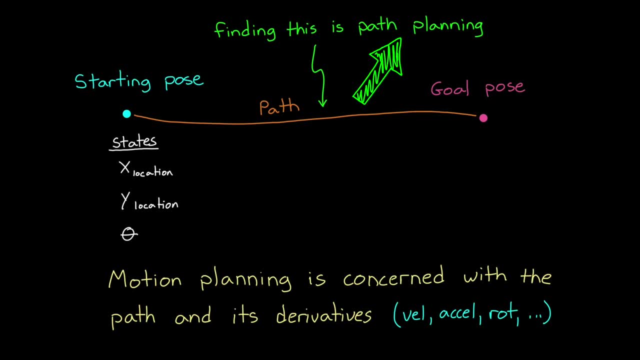 precisely how the robot moves through the environment. With path planning, we're just concerned with the path that it takes and not how fast it accelerates or moves through it. But even though you have three states, you're just lost in time taking into account parameters. 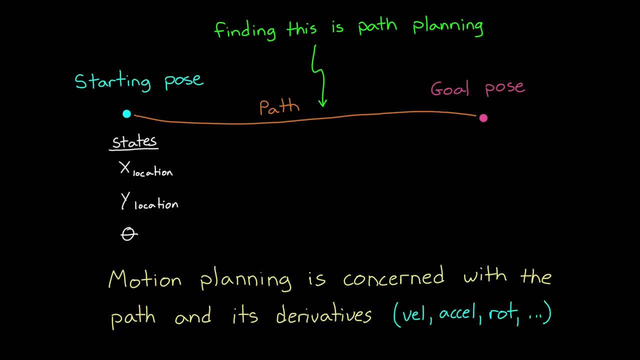 that have no relation. So if you move outside your training environment, to take into consideration what this could take to the robot you'd want to use, the implementation opens Now. the size of the pose vector depends on the specifics of your system and environment. Instead of three, 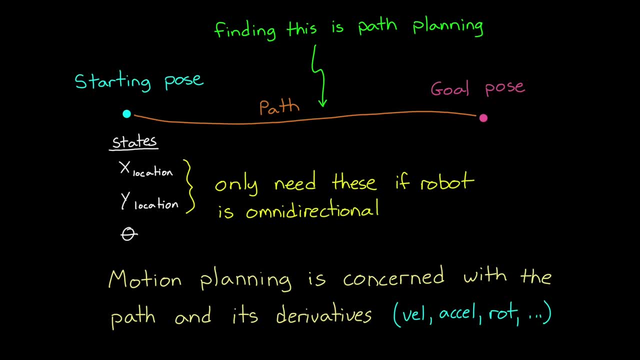 states, it could be just two x and y. if the robot is omnidirectional and orientation doesn't matter, or in the case of a robotic arm with multiple actuators, the pose could consist of dozens of states. now for this video. the examples i'm going to use focus on path planning and for a robot that 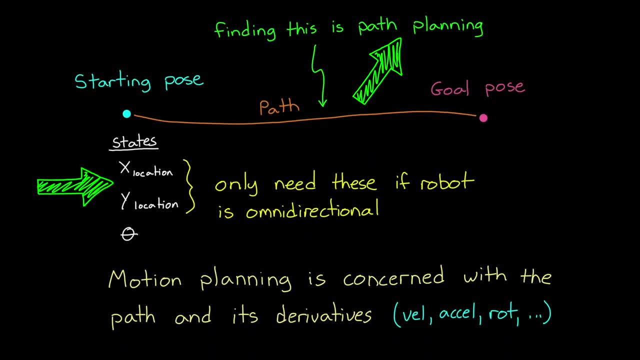 is omnidirectional, so just two pose states. this will simplify the explanation and hopefully you'll be able to see that these techniques can be extrapolated to higher dimensional systems. all right, let's get started with a simple map that's similar to the one that we generated in. 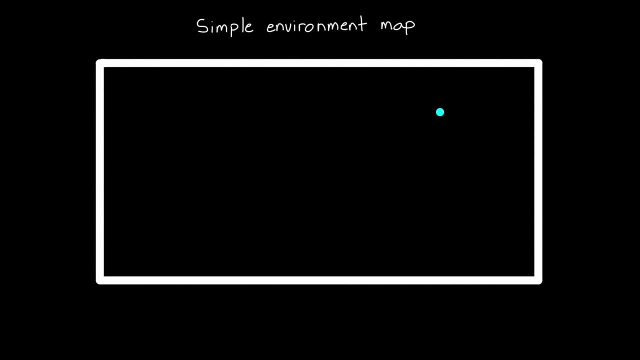 the last video. it's just a rectangle and assume that the starting pose is up here and the goal pose is over here. a minimum distance solution can be solved for directly by connecting the start and the goal with a straight line, as long as there's no obstacles in the way. now, if the robot moves, 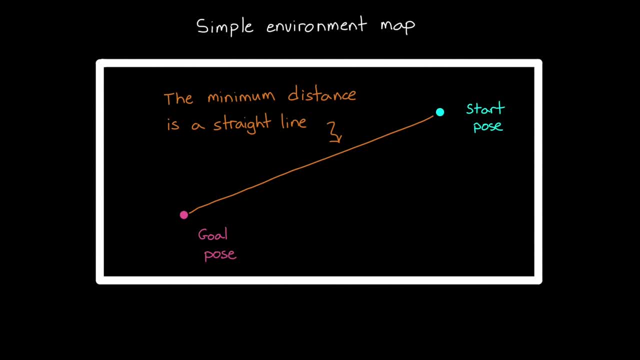 along the path, it will be able to see that it has the exact same position as the robot does. now, if the robot moves along the path, it will be able to see that it has the exact same position as the robot does. this path. it's going to reach the goal in the shortest distance possible. now, analytically. 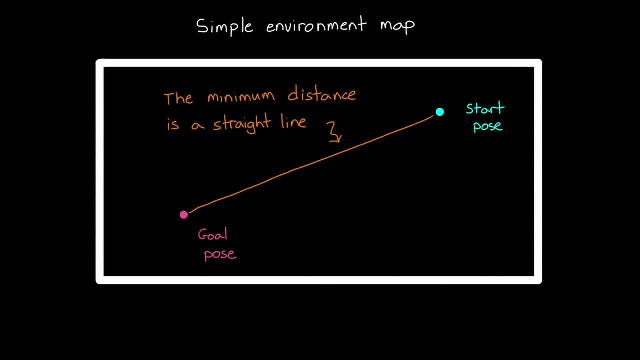 solving for the shortest path like this is trivial for our simple environment, and this type of solution could even work for environments with some obstacles and constraints as well. but for many problems, the obstacles and the dynamics of the system are too complex to generate an optimal solution analytically. so we approach it by solving the problem numerically and, as i said at the 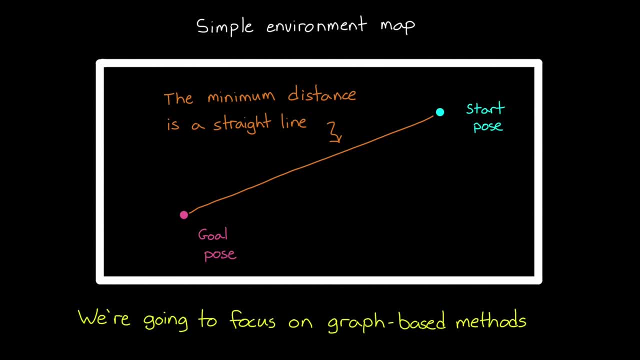 beginning of this video, we're going to focus on graph based methods to numerically find the path with the shortest length. before we get into any particular algorithm, let me show you the general idea behind graph based solutions with this simple map. graph based algorithms work by discretizing the environment, that is, breaking it up into discrete points or nodes, and then finding 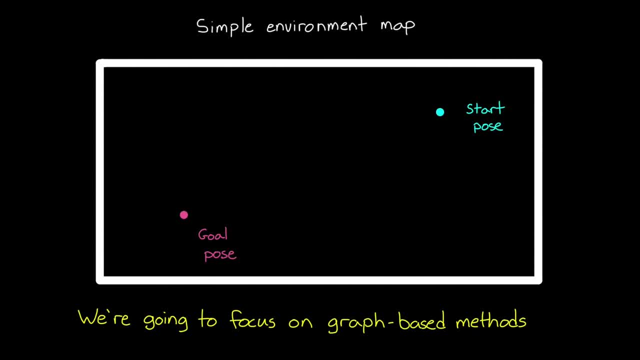 the shortest distance to the goal, considering only these nodes. let's approach this problem in a random way. the starting location is the first node in our graph and it has a cost of zero since we're already there. so i'll put a zero inside the node, then we can move in a 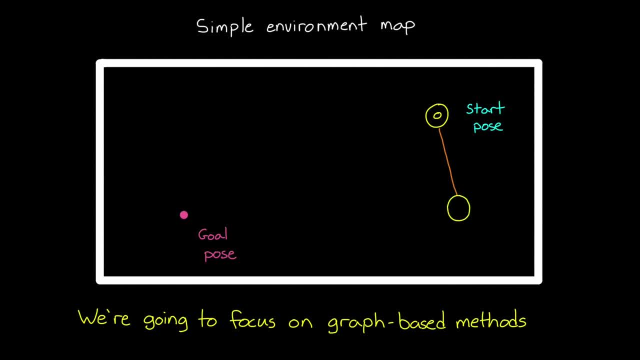 random direction and place a node in the graph at our new location. the edge between the nodes is how far we traveled and the cost of getting to this node is the length of that one edge. now we take another step in a completely random direction, place another edge and the starting location. 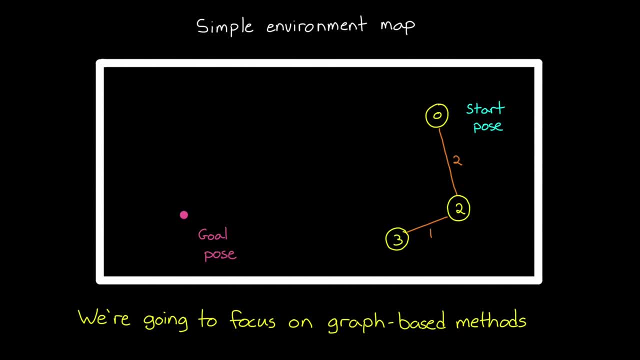 and the cost of this node is the total of three units, And we can continue to do this on sort of a random walk until we get to the goal, And the cost of this particular random path is 10 units. We've found a path that works. 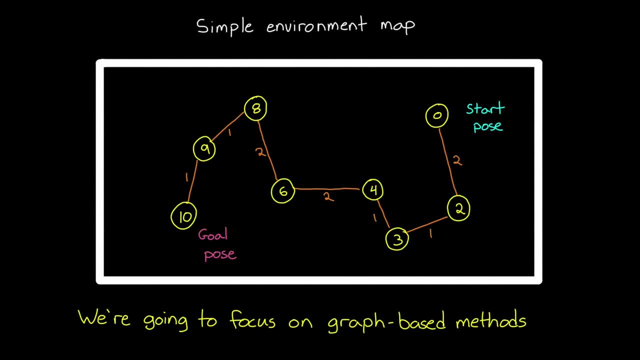 even though it's definitely not the shortest path. So we can start again taking a new random step and adding a node and connecting it with an edge and recording its cost. And if we happen to reach a node that we visited before, we can compare the cost between the two different paths. 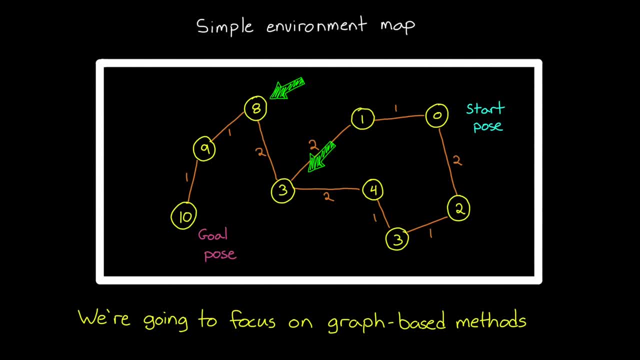 that we took to reach it and keep the smallest one. Basically, we're revising our estimate on how many units it takes to reach that particular node. We now have this graph of nodes or locations on a map and how much it costs to get to each node. 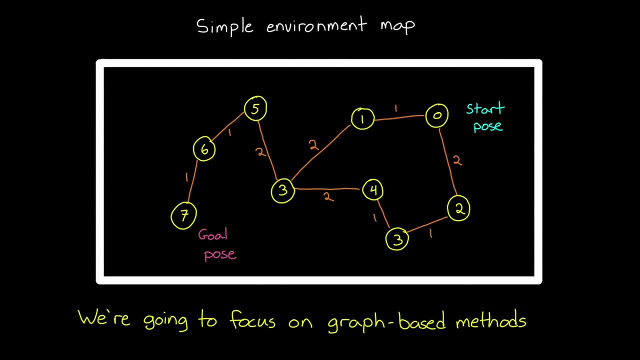 But we should recognize here that we don't actually need to build a fully interconnected graph, just a tree Which is a subset of a graph. A graph can have nodes connected in any way you want, but in a tree each node only has a single parent. 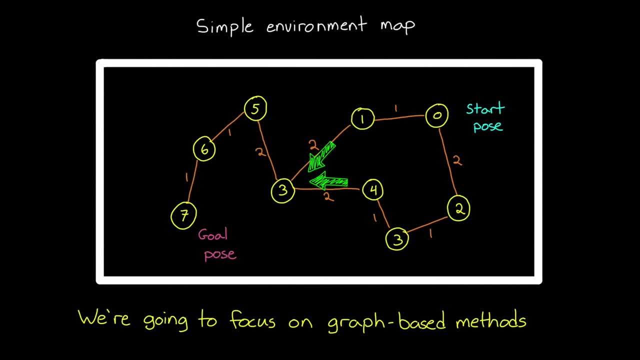 If you can get to a node two different ways, it doesn't make sense to keep the path that is longer if you're looking for the shortest path. So you can remove the edge for the longer path, keeping a tree structure. In this way, a tree would start at the location of the robot. 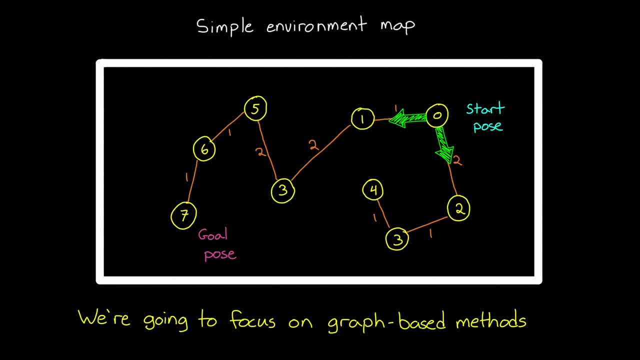 and the branches would venture out to other states, but never recombine Now to find a shorter distance to the goal. we can just keep randomly wandering the environment, updating the tree, until we find a branch that gets to the goal with a cost that is low enough. 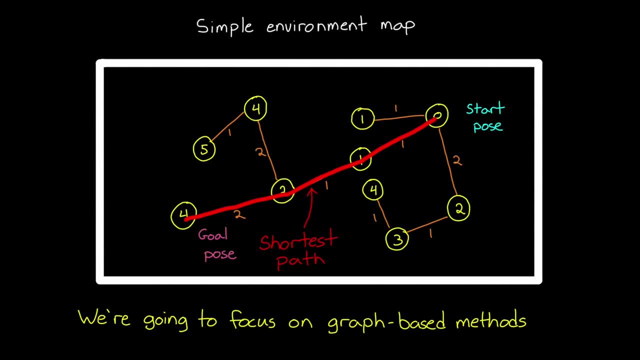 It doesn't guarantee an optimal path, but it will continue to approach optimal as the number of nodes go to infinity. Of course, building up a tree through random wandering is not the best solution, So this is where path planning algorithms come in. They provide more efficient ways. 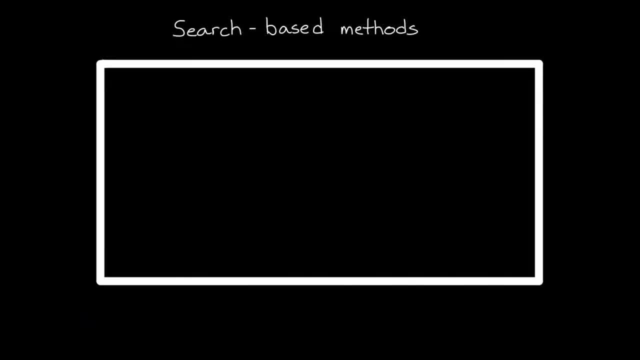 to build a tree. I want to start with the so-called search-based methods that build up the tree by adding nodes in an ordered pattern, And one way to accomplish this in practice is to start with a grid-based map, like the occupancy grid that we have. 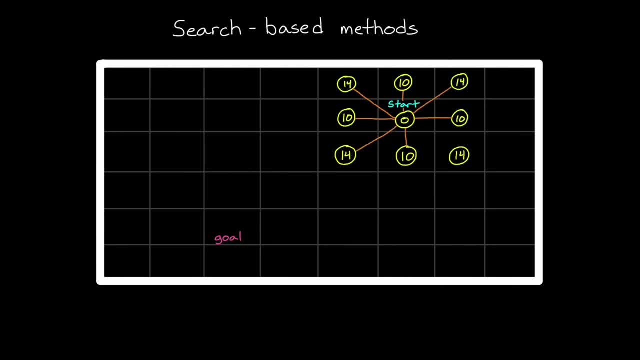 and go cell by cell and determine the cost or the distance the robot would have to go in order to reach that cell. Here I'm claiming adjacent moves are 10 units and diagonal moves are 14.. Now, this is similar to the random approach that we just did. 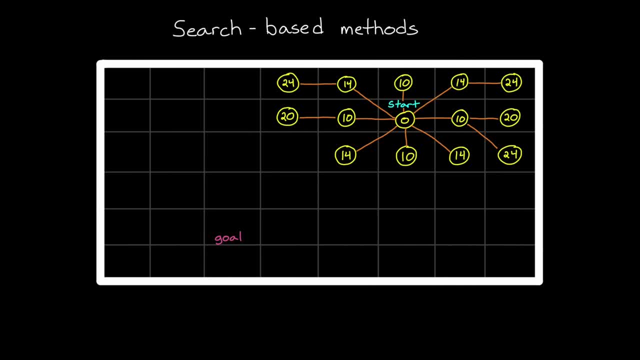 except we're methodically working our way through each cell and calculating the cost to reach it, And if it's the shortest path to that node, then we update the cost and the tree to reflect it. And once we've covered every single cell in the grid, 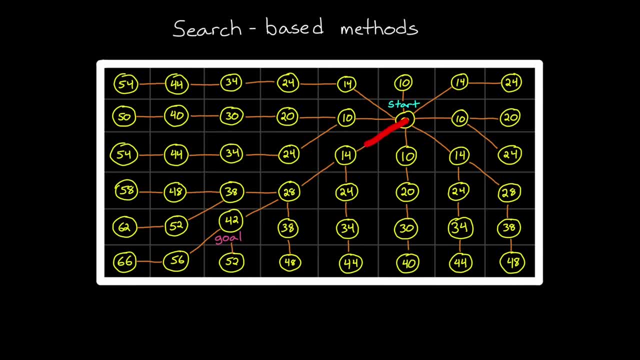 the optimal path is simply the sequence of cells that produce the minimum cost at the goal. This will produce an optimal solution, at least optimal at the resolution of the grid. But you can see that it would be computationally expensive, since it's kind of a brute force method of checking every possible node. 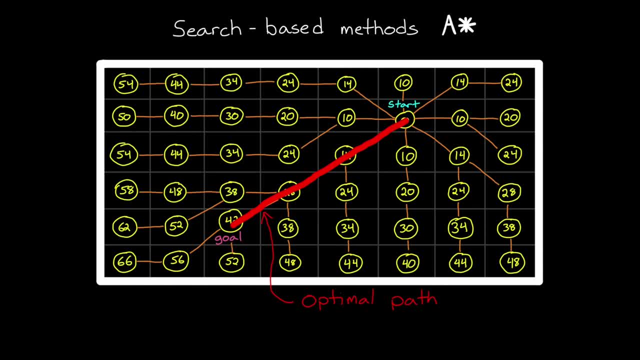 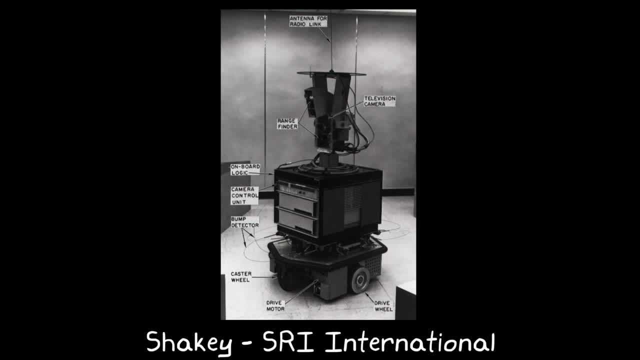 So to improve this, researchers came up with the A-star algorithm. This was in 1968, to give Shakey the Robot the ability to determine where to go on its own, which was a first for general-purpose mobile robots. This search-based method still adds nodes in an ordered way. 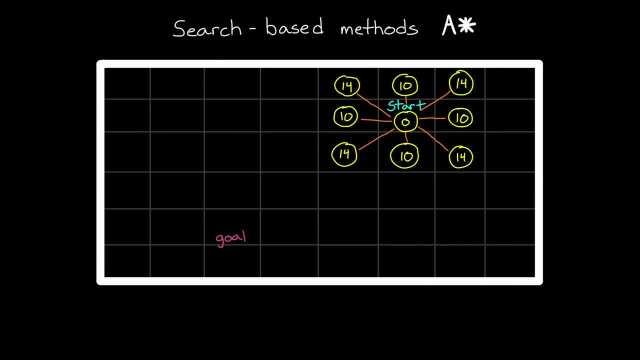 but it does so by prioritizing the nodes that are more likely to produce the optimal path and searching there first. It does this by keeping track of some other heuristic, like the straight-line distance from a node to the goal, in addition to the cost of the node. 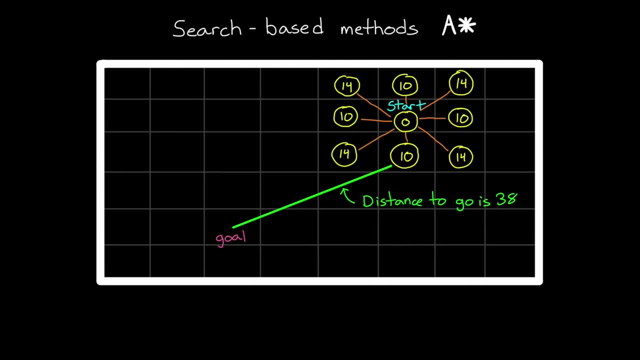 And the sum of these two numbers is the absolute minimum cost of the path. If there was a straight-line shot to the goal, then you could imagine how the total path length for, say, this node would be 48.. We've already gone 10 units and we have a minimum of 38 left to go. 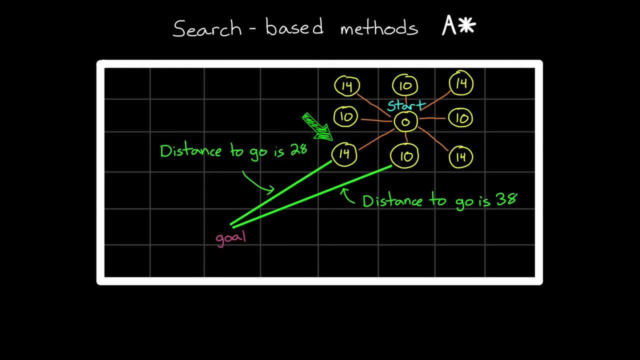 Therefore, this other node should be prioritized, even though its current cost is 14,, since there is the potential of only having 28 more units to go for a total of 42. It makes sense to keep trying this path. So in this way, A-star allows us to search through the nodes. 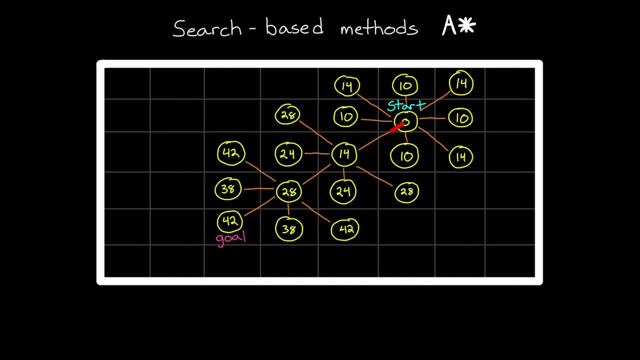 in a way that will get us to the goal without necessarily having to add every node into our tree. In fact, once we get to the goal, we know that we took the optimal path, since every node in our tree is the optimal path. 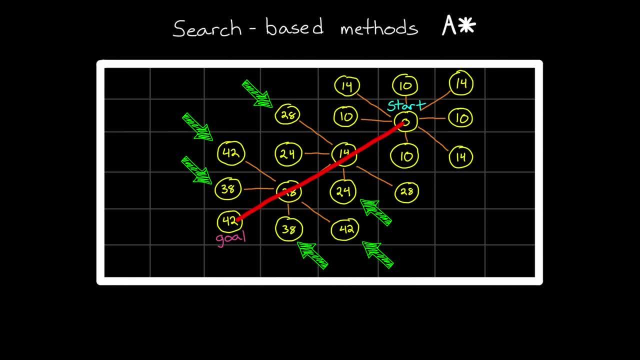 Every other path would have a cost plus distance to go that is greater than the path that we found Now. this was a fast introduction to A-star and I was going to make an animation that shows how this still works in the presence of obstacles. 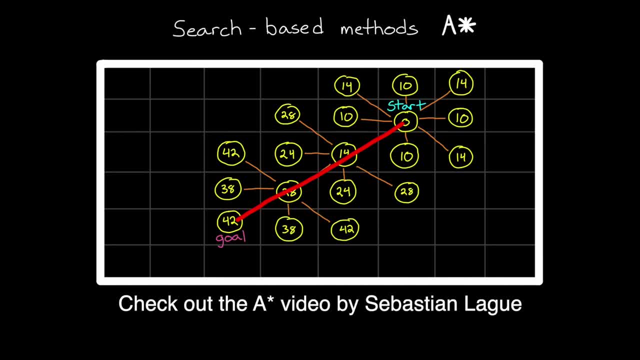 But honestly, I couldn't do better than what Sebastian Lague already has on his YouTube channel, which I've linked below. His video and animation on A-star is amazing and I recommend you check it out if you'd like to know more about this method. 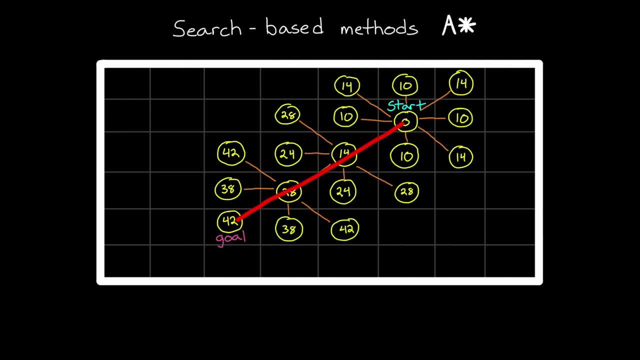 All right, So search on A-star. Search-based algorithms give us a way to build up a tree by adding nodes in some kind of an ordered pattern. But one problem with these types of algorithms- even efficient ones like A-star- is that they become very computationally expensive. 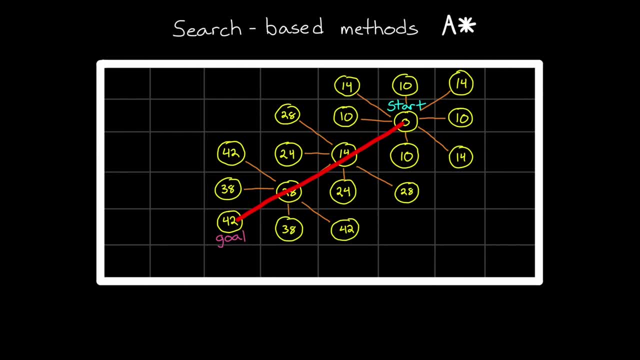 as the size and dimensions of the state space increases. You can imagine how the number of grid points grow exponentially as the number of dimensions increase, which can slow everything down. So they tend to not be used for high-dimensional state spaces. things like determining the path for multi-joint. 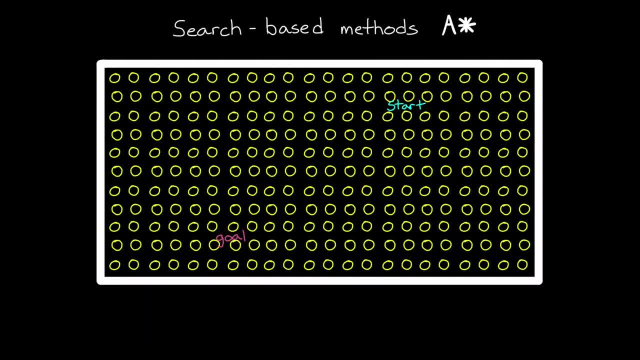 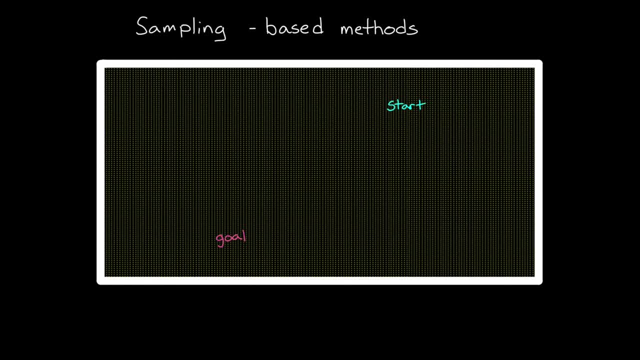 pointed robot manipulators, Or for really large, low-dimensional state spaces, ones that might have millions or more grid cells. This is where the so-called sampling-based algorithms are useful. To understand how sampling-based algorithms work, I think it's first helpful to realize that in our map. 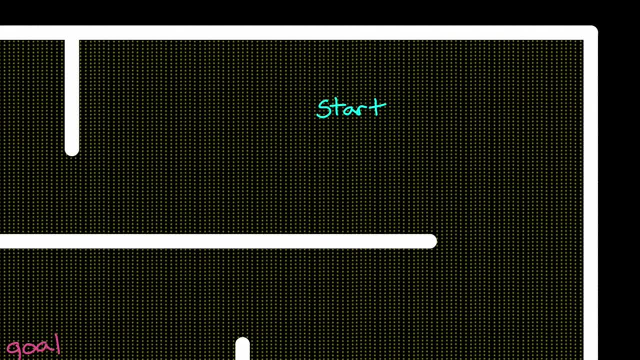 and probably most maps. there are sections where a path could continue in a straight direction for some distance before it needs to make a turn. With A-star we have to calculate every single grid cell between these two points, so multiple nodes in the tree. 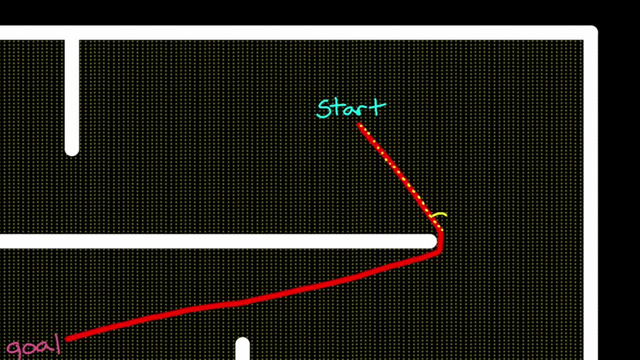 However, if we only checked the far distant node and there weren't any obstacles in the way, then we could calculate the straight-line cost for just this one node. This reduces the total number of nodes and therefore the total number of calculations. 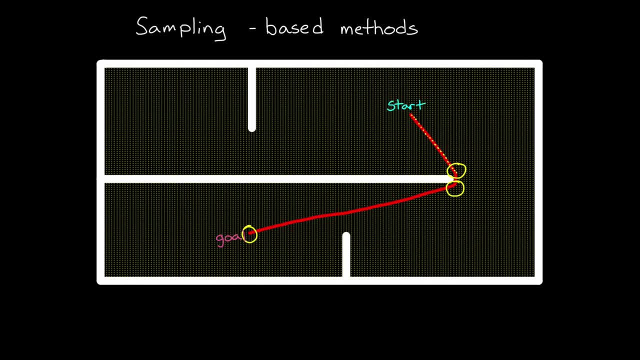 So the question becomes: how do we pick the location of these sparse nodes so that we still reach the goal? And one answer is to randomly select them Or sample them, hence the name. Now I know I said that randomly selecting nodes. 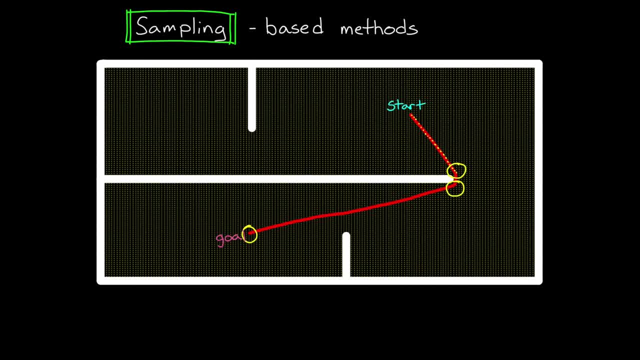 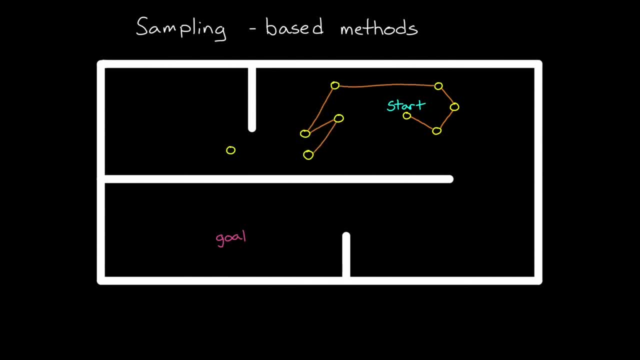 is not the best approach to build out a tree, but we're going to choose a random node location a little bit differently, Rather than extending the path through some kind of random walk, which could allow the path to circle back on itself and take a long time to explore in the direction of the goal. 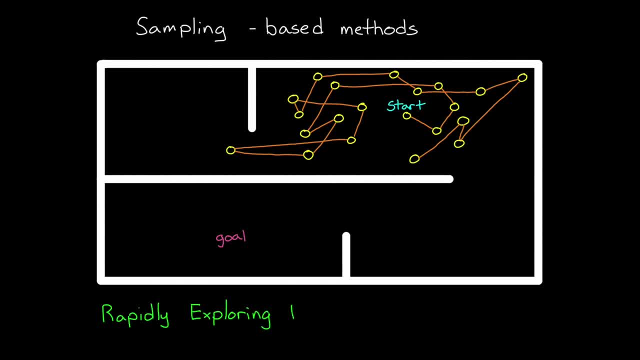 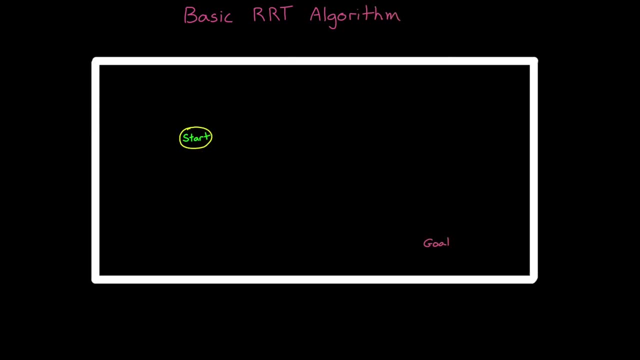 we're going to be smarter about randomization and focus on rapidly exploring random trees- RRT and a version of it that can approach an optimal solution called RRT star. Let's go into how the basic RRT algorithm works From the starting node. we need to place a new node in our tree. 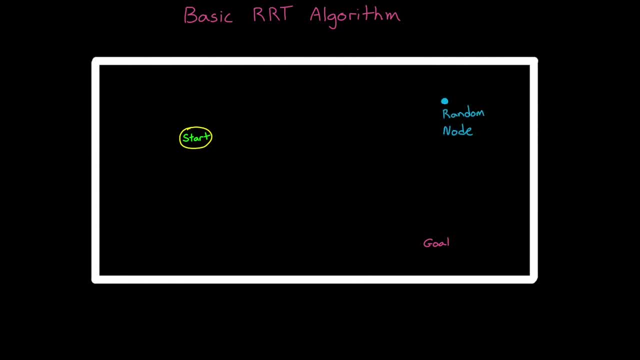 And RRT does this by randomly selecting a node anywhere in the state space. And once we have this random node, we want to connect it to the nearest node in our tree, which, since we're just starting, is the first node, But we don't want to place it too far away. 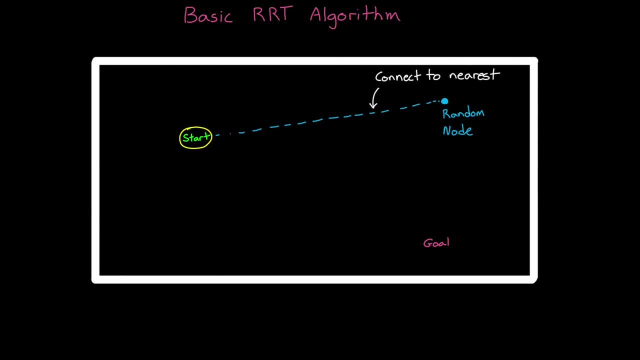 Because the chance of the path crossing an obstacle or just traveling too far in the wrong direction is greater with a longer edge. So we specify a maximum distance that the new node can be away from the nearest node. Now a quick aside. 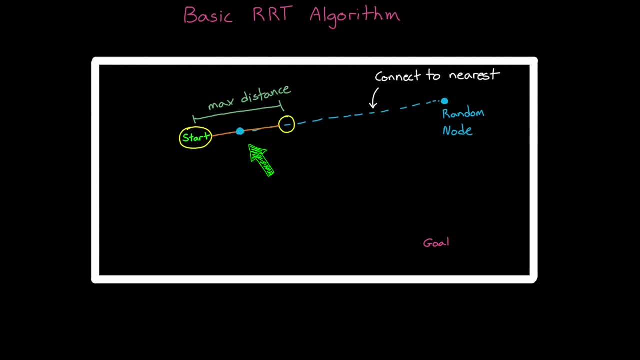 If the random node is closer than the max distance, then we just place the new node right there. Also, if there's an obstacle between the nearest node and where we want to place the new node, then that one's just ignored completely. nothing is added to the tree and we move on. 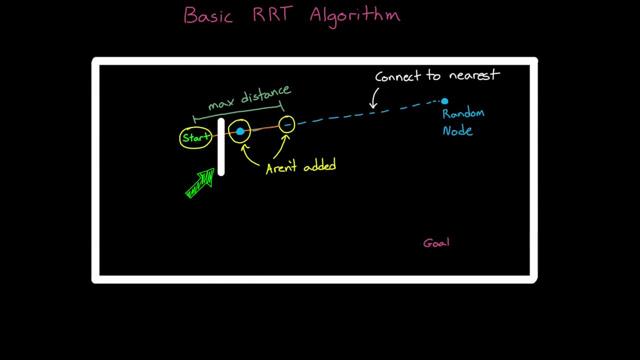 We don't want the tree from attempting to cross through any walls or other obstacles. Okay, let's move on. We randomly select a new node and find which existing node it's nearest to. Again, this happens to be the starting node. 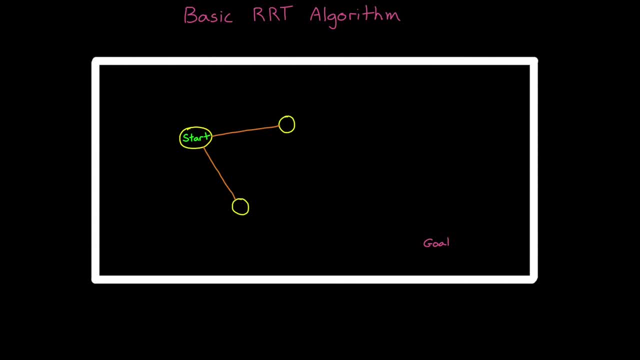 So we already have two paths in our tree and both are venturing out into different parts of the state space. A new random node, and again we connect it to the nearest, which is growing one path even further into the open space. This is why the algorithm is called. 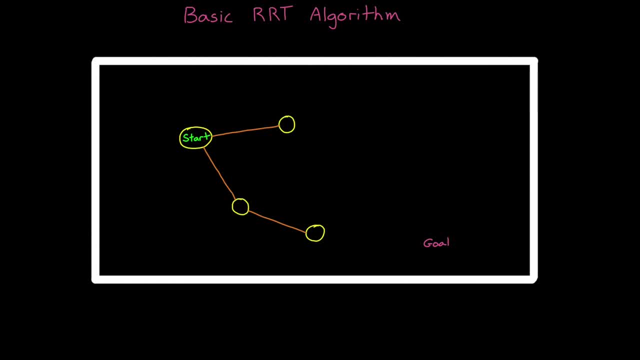 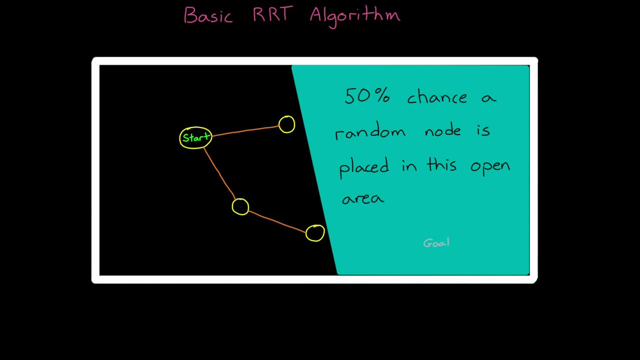 Rapidly Exploring Random Trees. When there are large unexplored areas like we have, then there's going to be a good chance that a random node is selected in that area And this has the effect of adding new nodes in places that cause the paths. 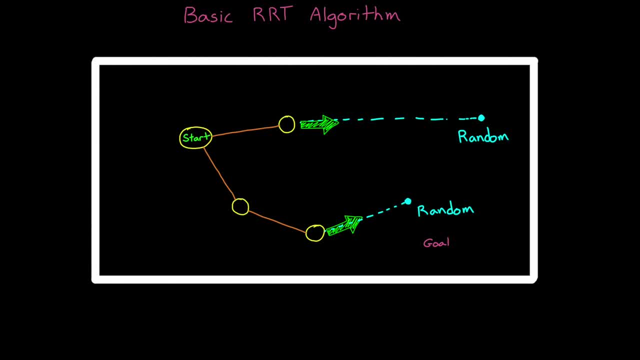 to venture into unexplored areas quickly at the beginning, Hence rapidly exploring. And a random node that is in a direction opposite of the goal doesn't affect the path that's on its way to the goal, since a different node will be in the direction opposite to the goal. 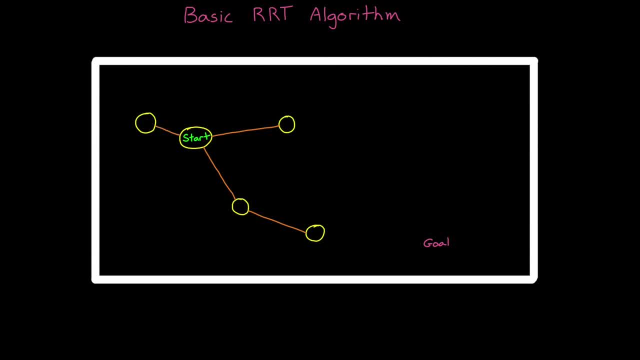 In this way, one path is always rapidly making its way towards the goal and the others are rapidly making their way into other open areas of the state space. And then, later on, as the unexplored area starts to fill up, the random node's selection tends to just fill the tree out with more branches. 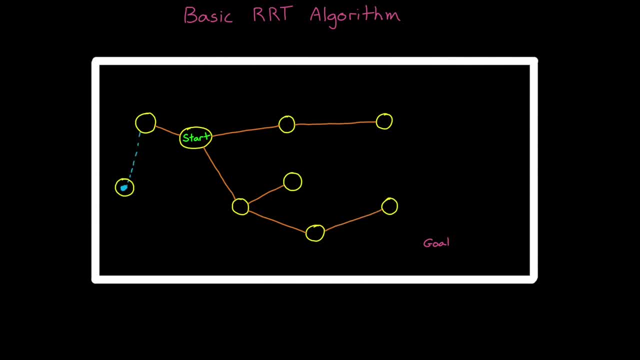 Now we can continue doing this process until the path gets to within some threshold of the goal. At that point we have a viable path, albeit probably not. It's probably not an optimal one, since this method tends to zigzag as it makes its way. 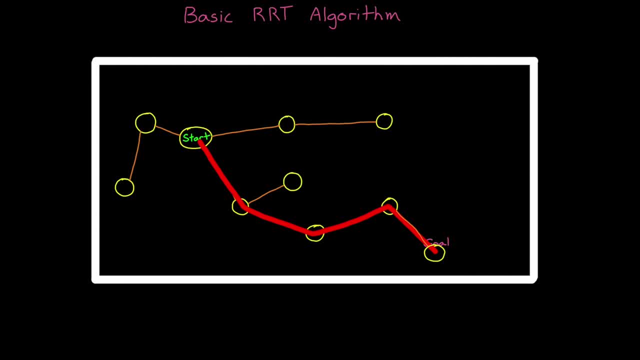 But we did find a solution And, importantly, a solution that is likely using fewer nodes than would have been necessary for A-star, since the nodes can be spaced further apart. Again, we set that with the maximum connection distance. Now RRT can work really well for situations where you're just looking for a valid path. 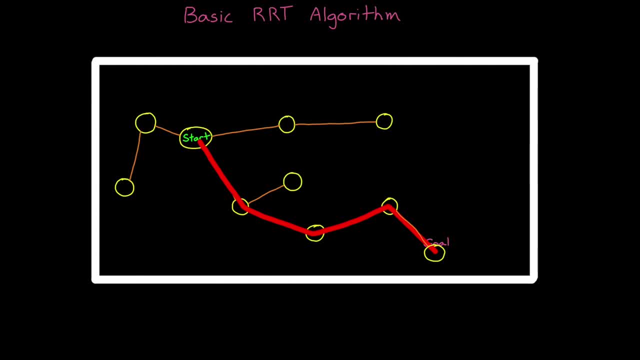 and not necessarily the shortest distance, As long as the start and goal nodes are reachable, this method is guaranteed to find a path as the number of samples approach infinity And, in most cases, a much, much smaller finite number of samples. 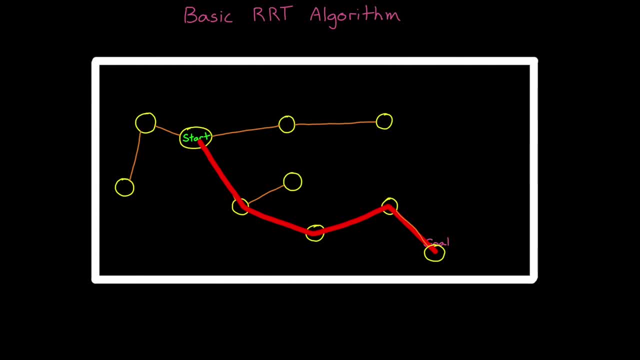 Now, if we do want a solution that's closer to optimal, we have to add some additional steps into the RRT algorithm and we get RRT-star. For RRT-star, the node selection process is exactly the same. We choose a random node, find the nearest neighbor. 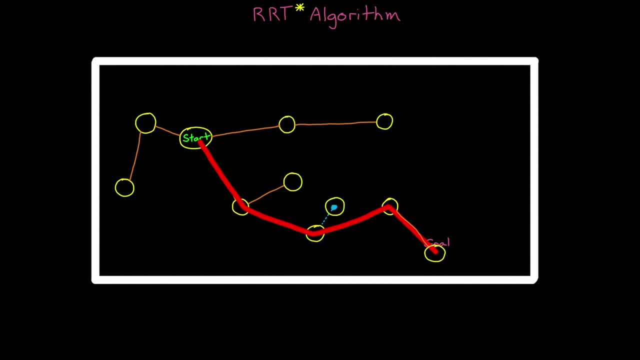 and if there's no obstacle in the way we place a new node, at the random node or at the max connection distance, whichever is smaller. The difference, however, comes from where we connect this node to the existing tree. We don't necessarily connect it to the nearest node. 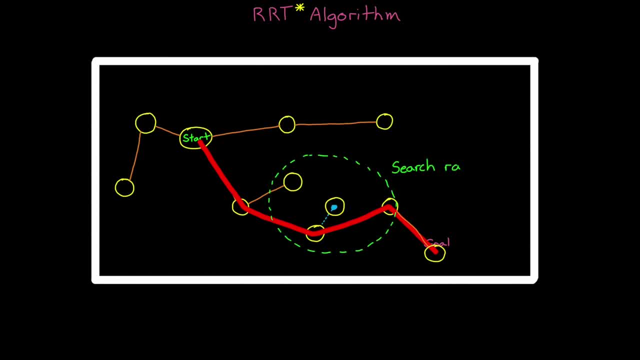 Instead, we check for other nodes within some specified search radius and determine if we can reconnect these local nodes in a way that maintains the tree structure but also minimizes the total path length. So here I'm, connecting it to this other node. 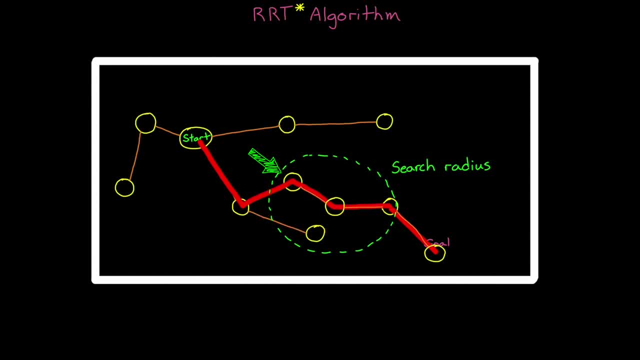 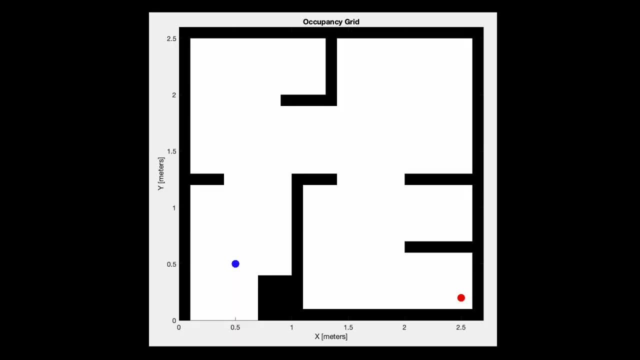 since that's going to produce a shorter path back to the start. Let's watch RRT-star work with a slightly more complex environment. Here I'm using MATLAB to do the visualization and the RRT-star function. from the navigation toolbox At the beginning you can see that it's rapidly exploring the environment. 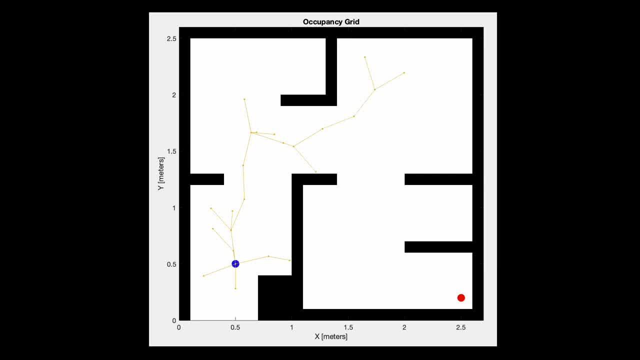 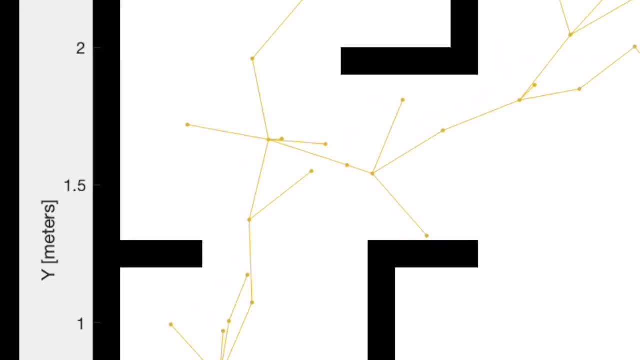 and doing so with just a couple dozen nodes. So far it's not different than RRT. but let me pause it right here. This next node is going to appear here. If this was RRT, it would connect that node to this one, since it's nearest. 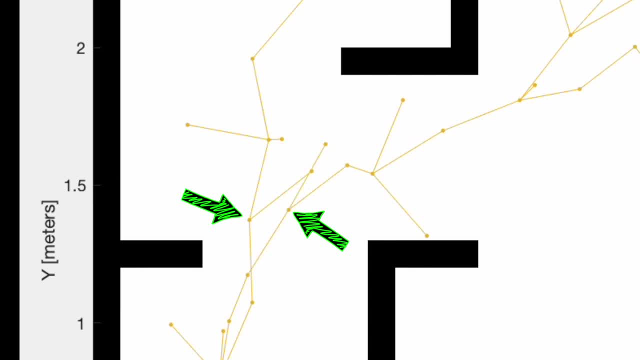 But watch what happens. That node appears and it's connected all the way down here, since that's a shorter path back to the start, And it reconnected some of the other nodes within the search radius, So RRT-star is always trying to shorten the paths. 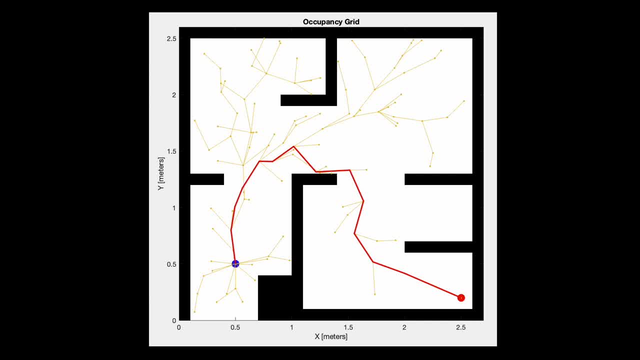 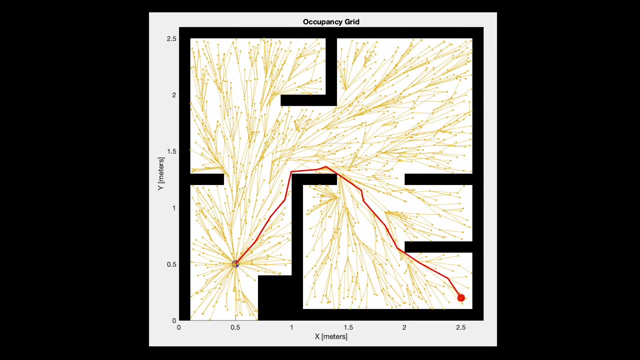 Let's continue Here. it reaches the goal and, just like with RRT, the path is a bit zig-zaggy at first, But as we continue adding more nodes and the existing paths are reconnected, you can see how they get refined over time, becoming shorter and straighter. 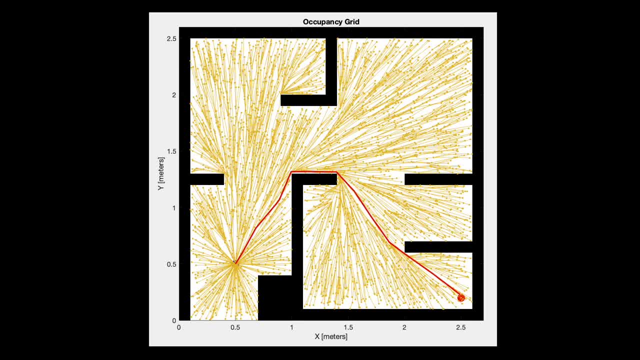 We can stop adding nodes whenever we're happy with the result. Now, not only do we have a near-optimal path to the goal, but our tree has generated near-optimal paths to anywhere in the environment, At least as long as the environment doesn't change. 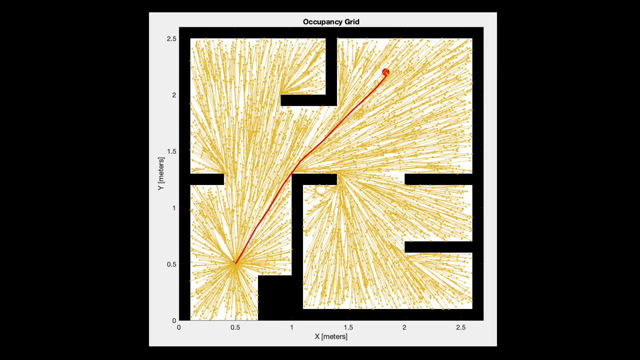 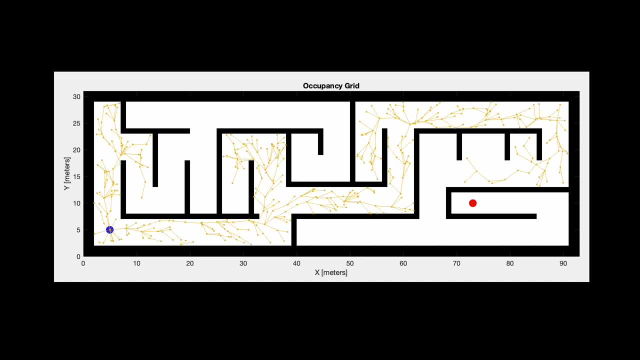 And this is the power of RRT-star. Now again, this was a super-quick introduction to sampling-based algorithms and I've left better sources of information in the description of this video. But that's where I'm going to leave it for now, with just the briefest of introductions. 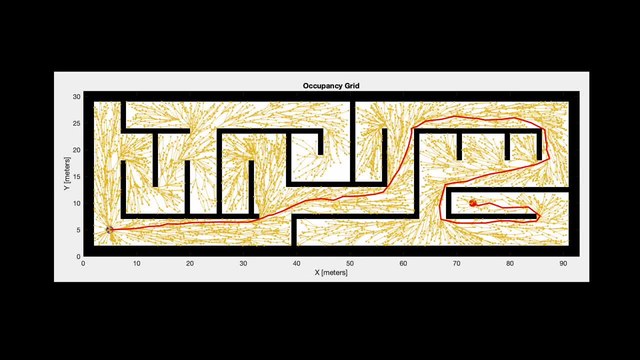 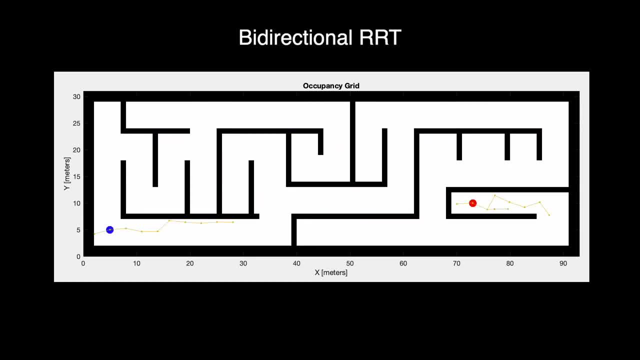 The idea here was not to tell you everything you need to know about path planning, as there's dozens of variations of just RRT alone, But hopefully you have a sense of how a tree can help you. RRT can help us plan a path through an environment. 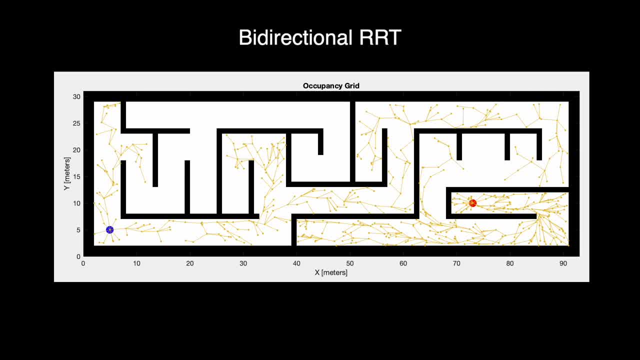 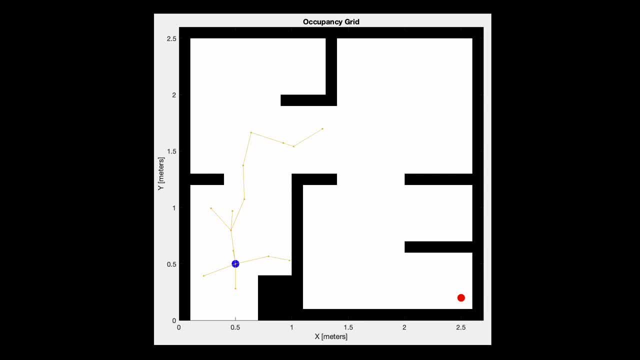 And some of the search-based and sampling-based ways we can approach building that tree. In this video, we dealt with planning a path through a static environment. However, often other objects and obstacles are moving through the environment as well, And planning algorithms need to react to those changes.